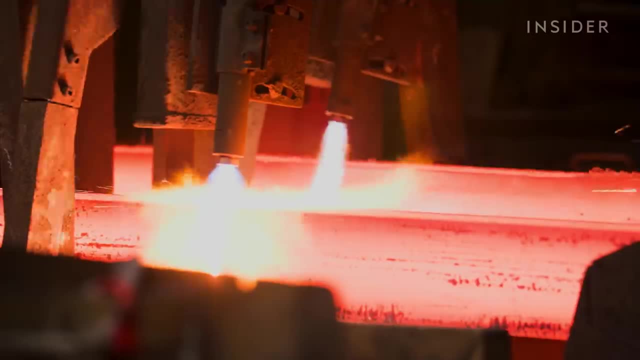 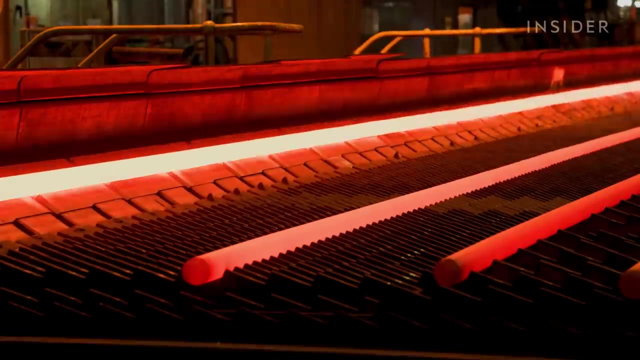 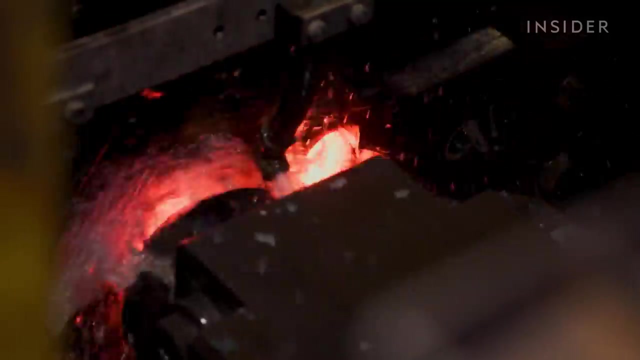 We use electricity, much like a large welder, to mine new iron. We melt that steel. Other processes adjust the steel's chemistry and strength. Molds shape the liquid steel into bars. The company sells some of these, but most are forged into a ball shape. 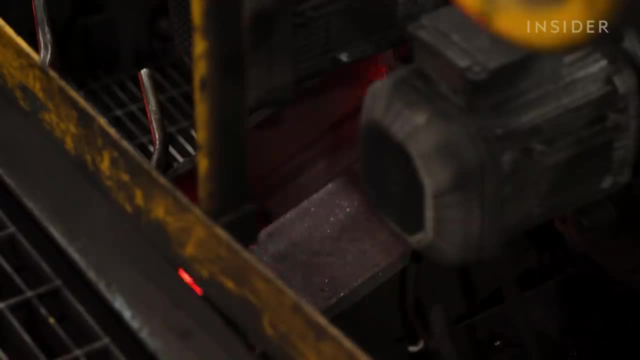 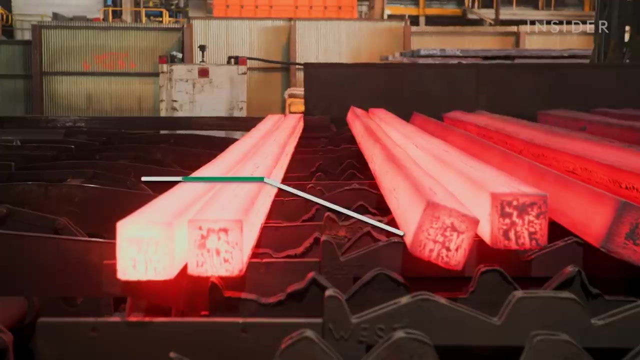 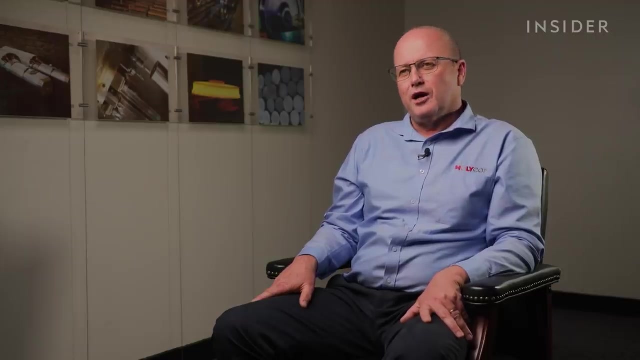 They're sold to copper and gold mining companies, which use them inside giant rotating mills to crush ore. Molycop says all of its products are made from 93% recycled materials, though Insider could not independently verify this. We want to push that as close as we can to 100%. 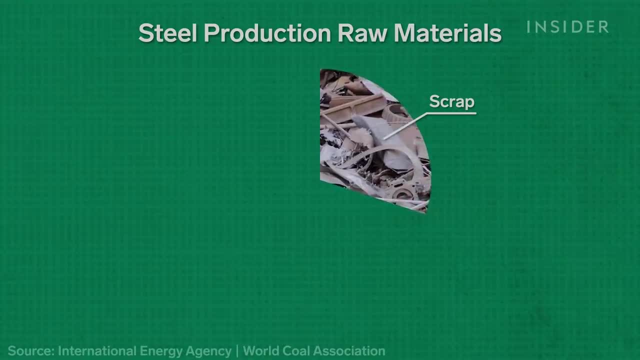 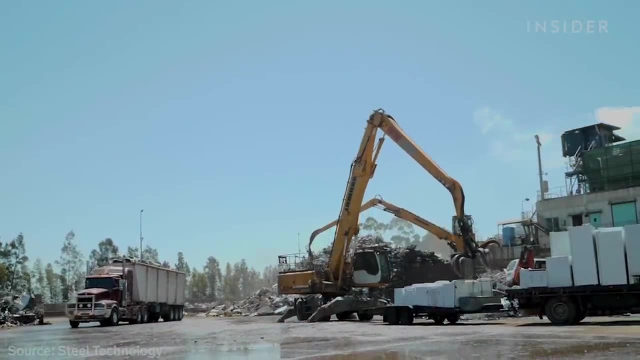 About a third of the steel made around the world each year comes from scrap. Nearly all the rest is new steel created from iron ore. Recycling is better for the planet and is usually cheaper, So why are we still making so much of it from scratch? 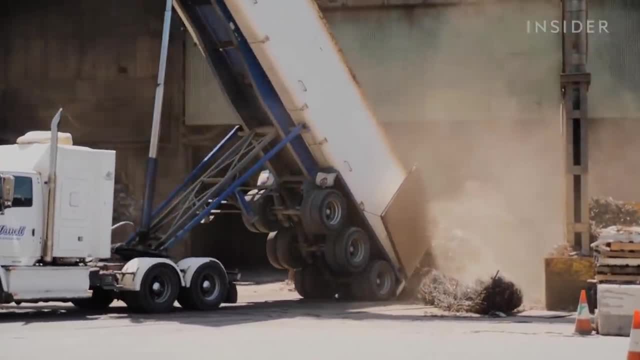 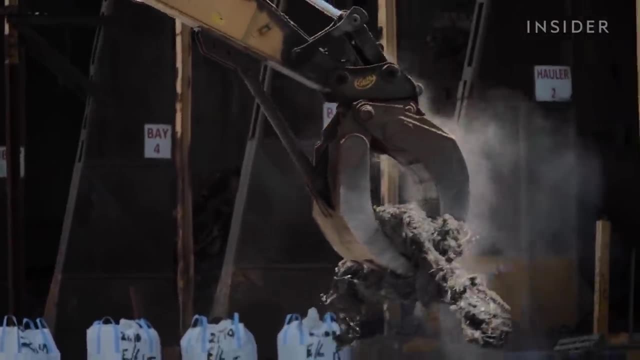 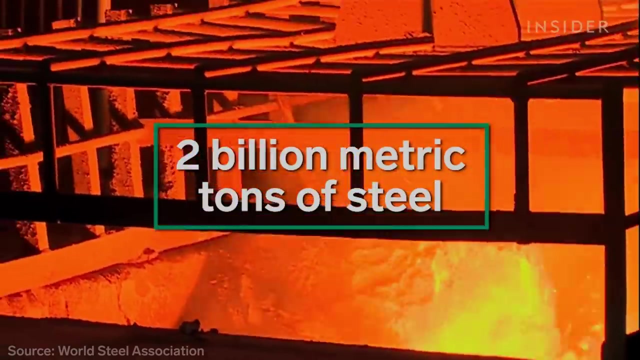 Because the world needs more steel than scraps can provide. It's really limited by scrap steel supply. The total demand for steel means that we'll still have to mine iron ore In 2020, the industry churned out almost 2 billion metric tons. About half of that went into buildings and bridges that won't become scrap for a long time, And scrap doesn't always end up in the hands of recyclers. In 2018, 7% of all the waste sent to US landfills was made of iron or steel. 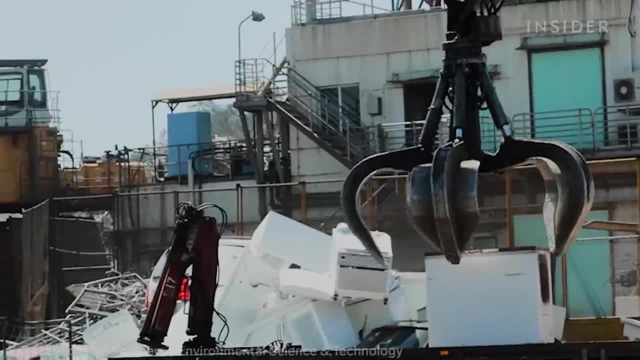 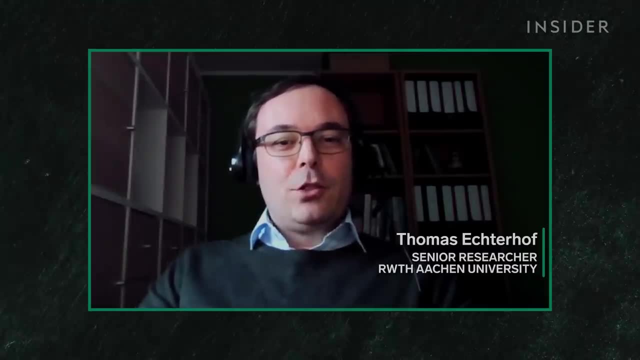 Plus, some experts say that purely scrap-based steel can't be used for everything. The main problem with scrap is that you always have some impurities in there which reduce the strength. With demand for steel on the rise, it's estimated that within the coming decades, 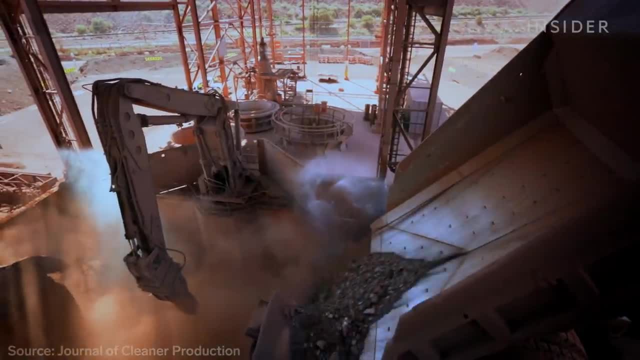 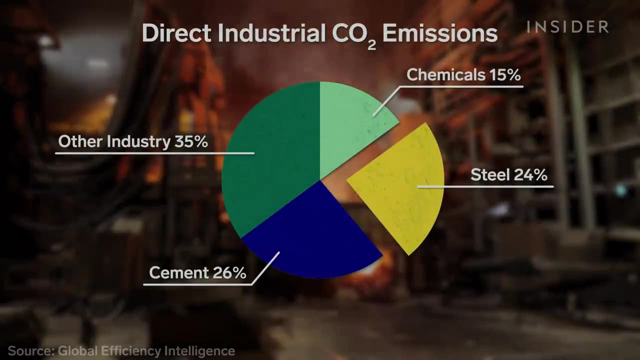 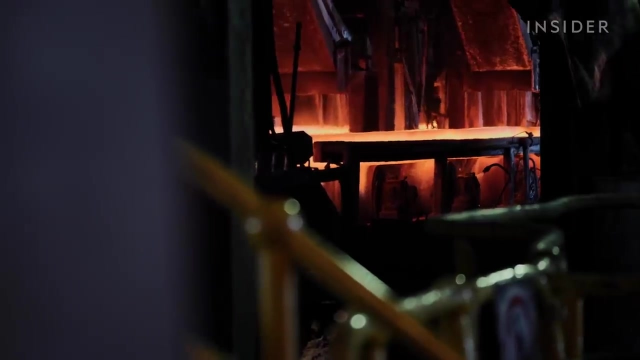 at least half of it will still have to be made from iron ore. That's a big issue for the climate. Steel is responsible for about a quarter of all industry-related greenhouse gas emissions. Most of that comes from cooking it up from scratch, But recycled steel is part of the problem too. 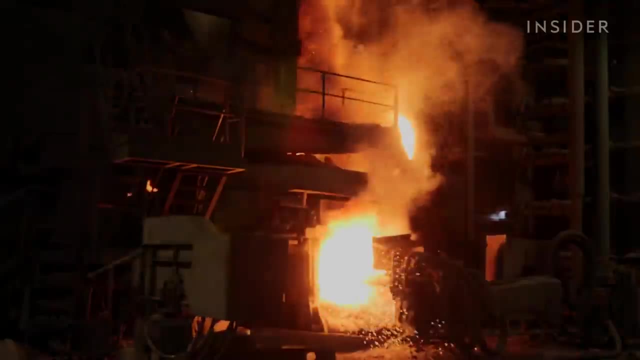 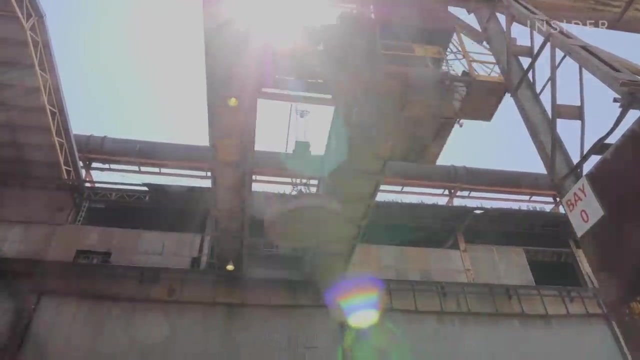 Melting scrap in a furnace uses a lot of electricity. Since 2020, Mollicop's plant has gotten over half its power from renewable solar and wind. Supporting the generation of renewable energy seemed a natural step to make and the right thing to do. 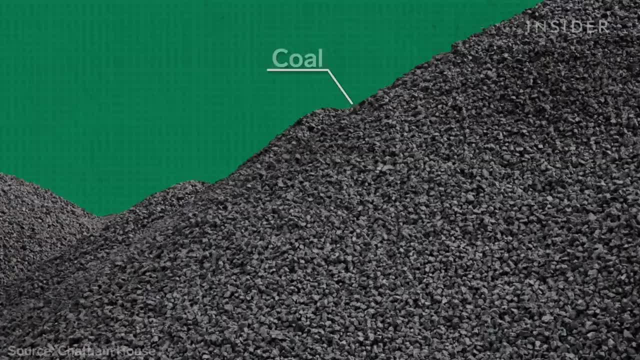 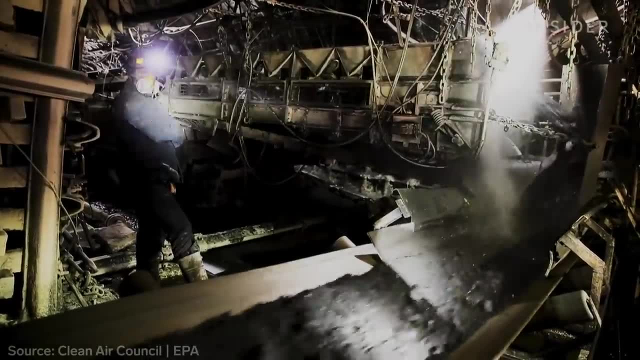 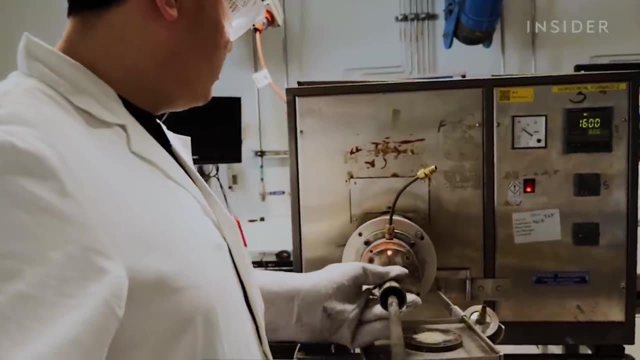 But even recycling usually requires coke, which is coal that's been baked for hours until it's almost pure carbon. You can't make steel without carbon, But mining coal and turning it into coke also uses lots of energy and creates air pollution. Mollicop is looking for other options.